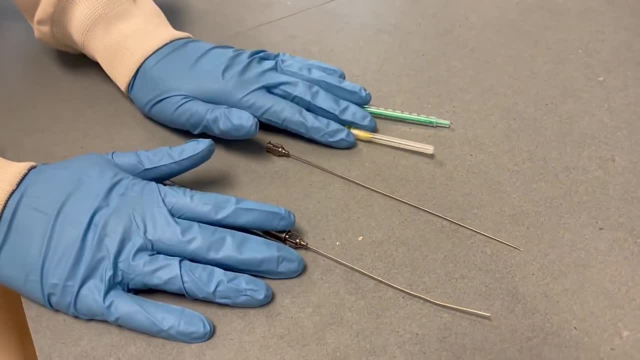 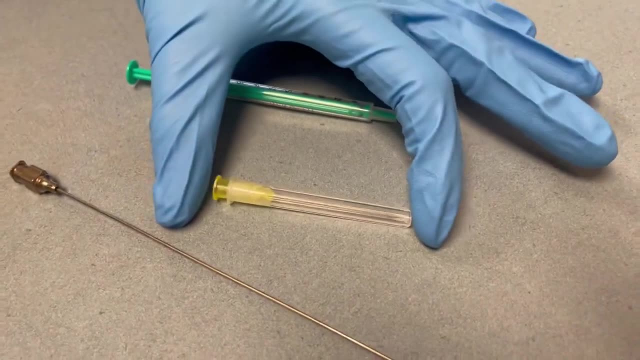 Disposable needles are convenient, since they're always clean and sharp, but since they're polypropylene, they can't be heated in the oven and we can't ensure that they're always moisture free. So we have stainless steel needles that can go in the oven. 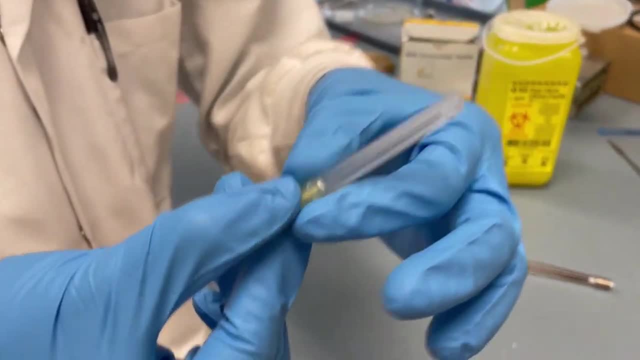 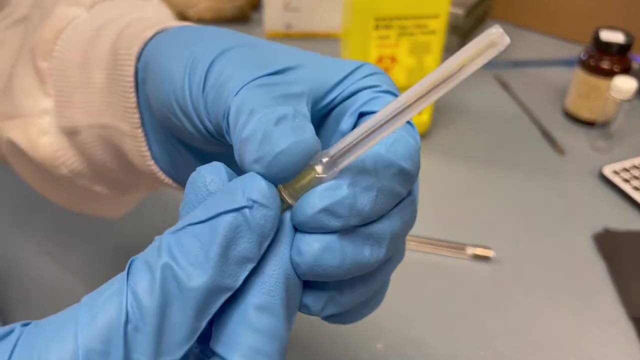 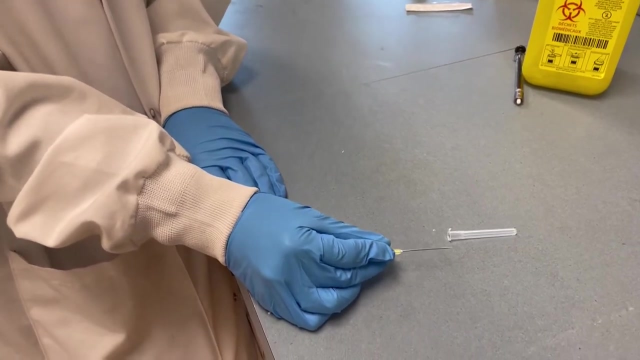 So when uncapping needles, you shouldn't apply excessive force, because when pulling the cap off, it might cause your hand to come back and result in accidental stabbing. Instead, you want to lightly twist the cap and that'll cause it to come off. So needles shouldn't be recapped, but if you must do so, you want to use the scoop method. 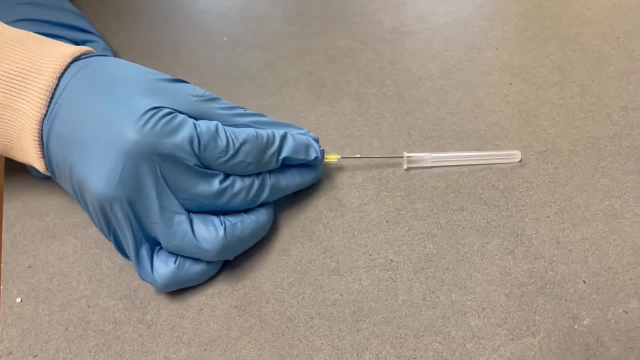 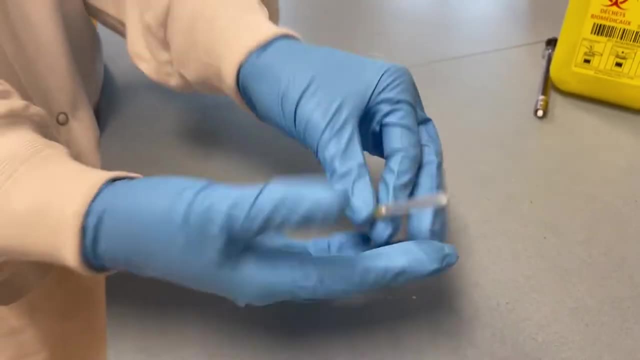 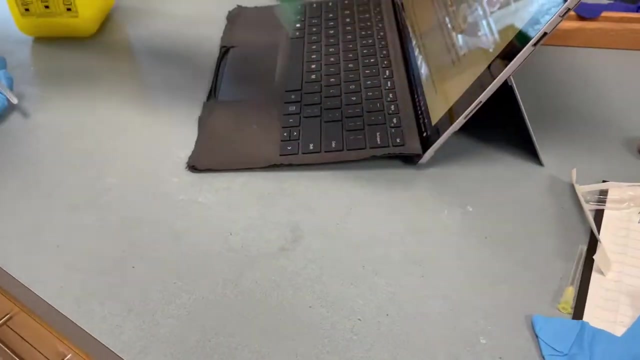 which is where you come at the cap at an angle, insert most of the needle in there until you can flip it back up and tighten the cap on there. And now to dispose of these, you can just toss them in a sharps container, but if they are on one of these, it has a little thing in here where you could stick the needle in. 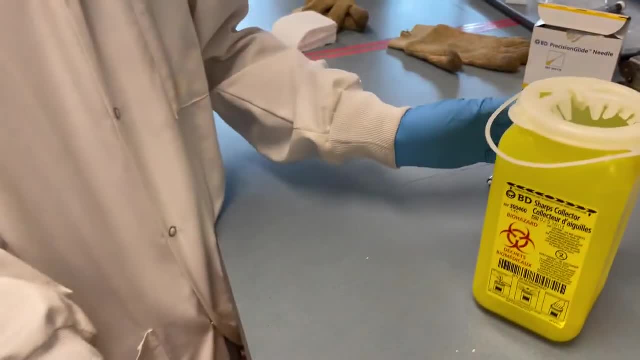 push up and then pull it out. So needles shouldn't be recapped. but if you must do so, you want to use the scoop method. it comes off on its own When you have the lure lock needle on a syringe and you want to remove the cap. 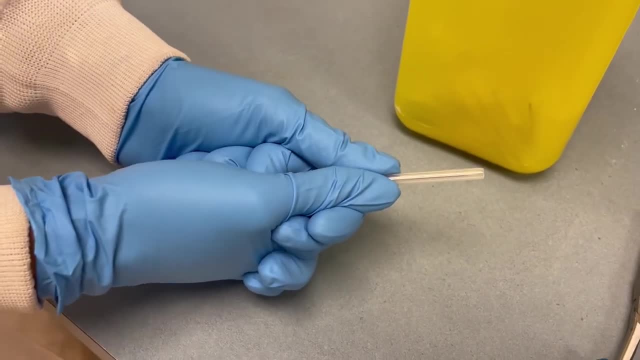 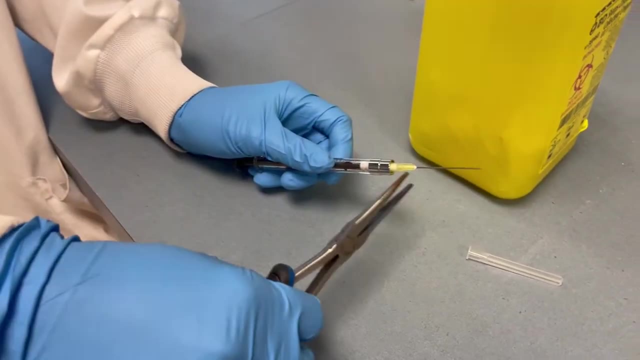 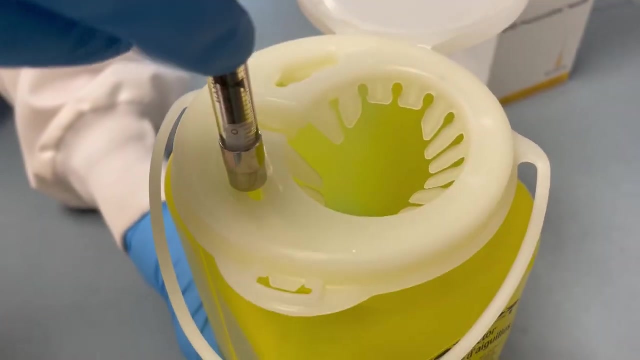 hold it firmly in one hand or both and remove the cap with both thumbs. If you're having difficulty doing that, you can also use a tool to help you remove the lid And to dispose of these needles. you can insert them into a slot at the top of the sharps container. 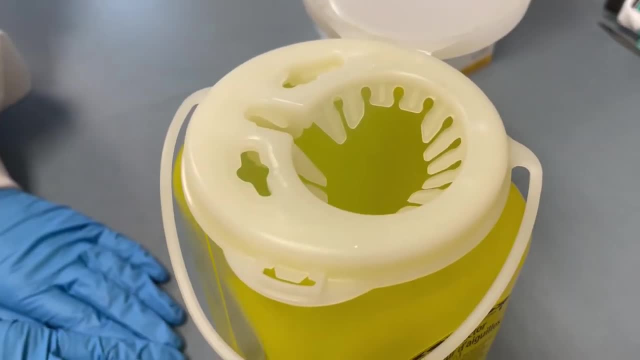 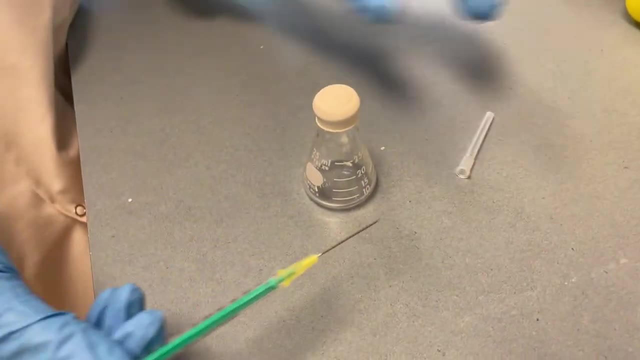 and just toss them in, Twist them off and then knock them right in. When using a needle with a septum or a shear seal bottle, you want to try and aim for the middle of the septum, as that's going to be the thinnest and most easiest to puncture through. 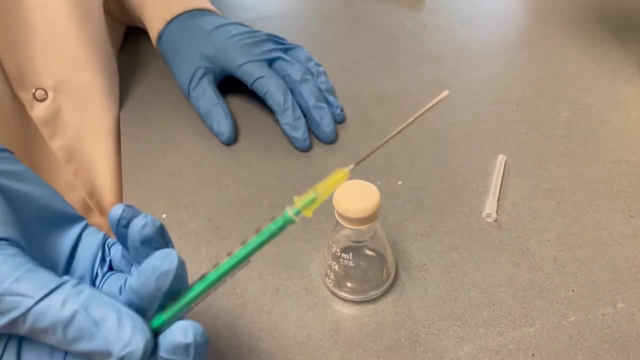 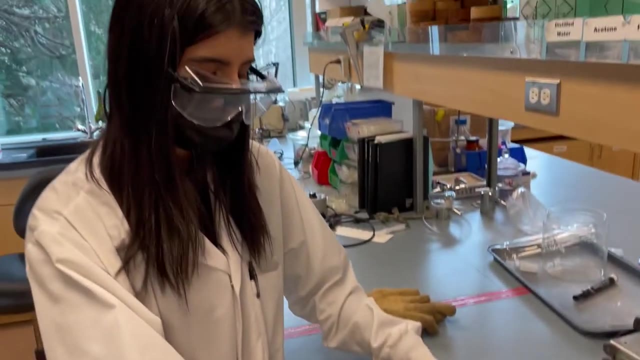 You just want to go in like that and to pull out. go slowly and it'll come right out. If you're going to store needles outside of the oven, you want to place them in a styrofoam block. Both can go in there. 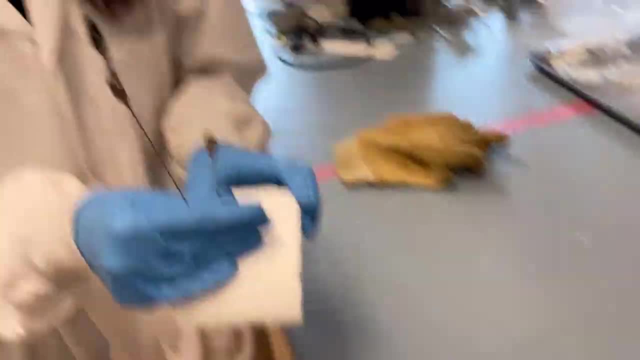 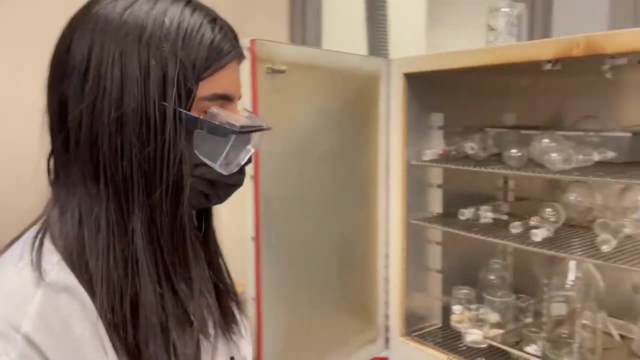 These ones can just be disposed of after use, and to store these in the oven, they should be kept needle down in a beaker to prevent anyone from poking their hands.